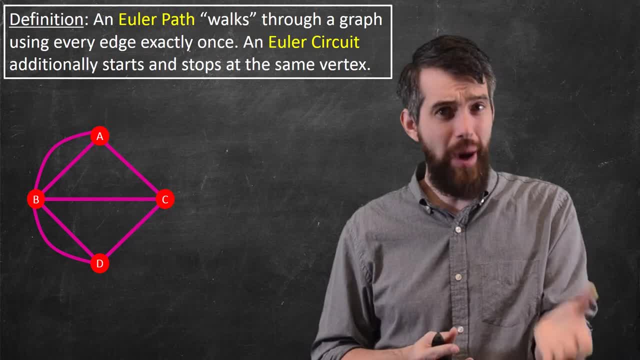 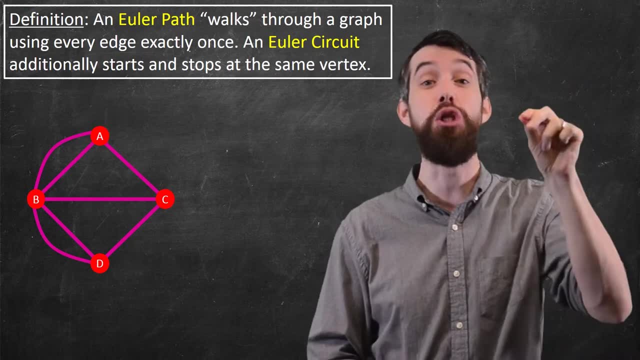 That is an Euler path And an Euler circuit is the same idea, the same. everything has to be hit once, but you start and finish at the exact same vertex, So it makes a loop, and then we call it an Euler circuit Instead of an Euler path. that might start somewhere. 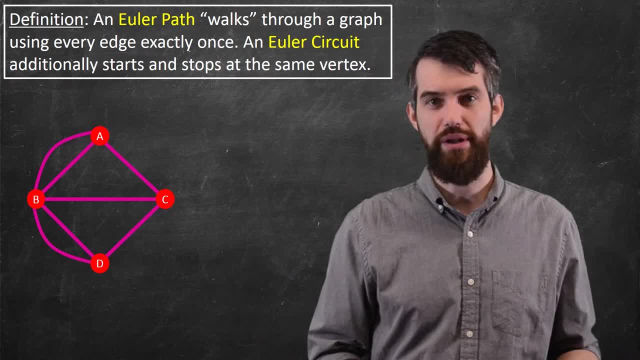 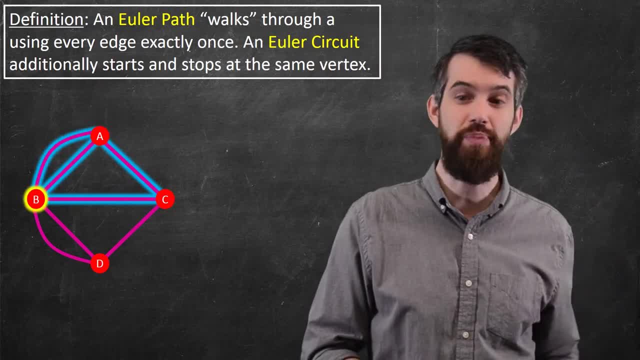 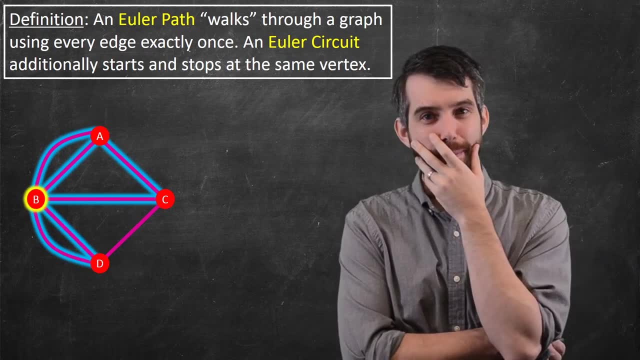 over to b. maybe I go back up to a, I go back down to b, I go down to d. here I go, maybe I don't know, back up to b. But then I have a problem, Because while I have gone along, 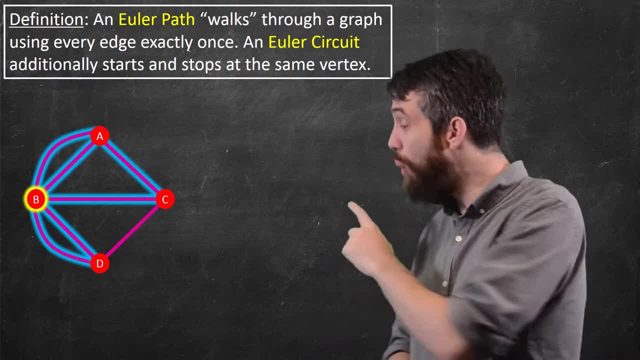 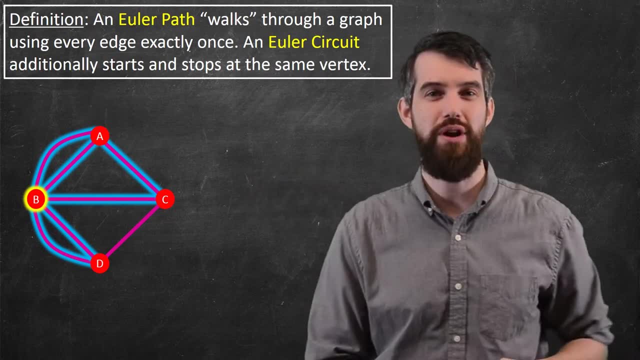 and I've used up almost all of the edges exactly once. there's still one edge that's missing, this connection between d and c. But how do I get there? Because right now I'm hanging out over at b And b's got every one of its five different edges. that leaves from b is 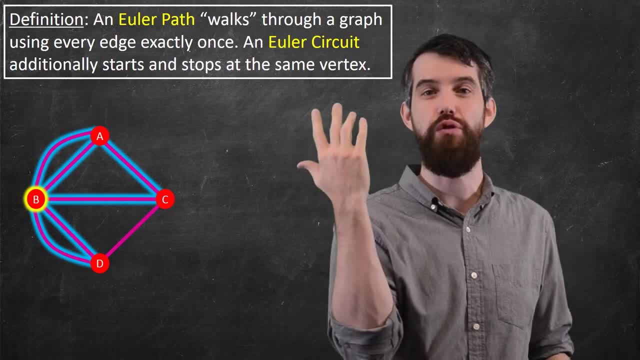 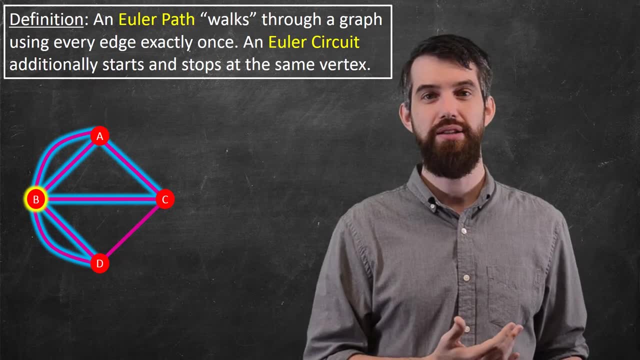 already being used. it's already gotten highlighted. I've done my Euler path and walked over them once already. So if I wanted to get down to d to c, I'd have to go over an edge. I've already done So. in other words, I can't actually get there via an Euler path or an Euler circuit. 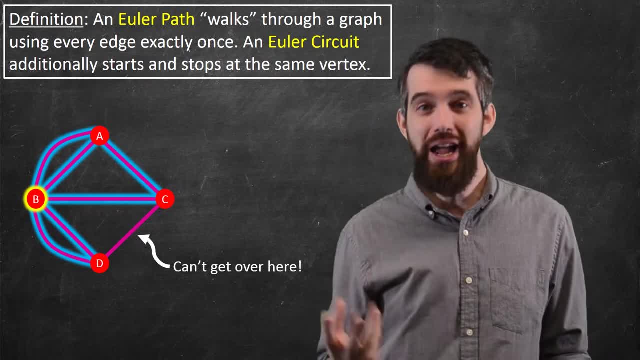 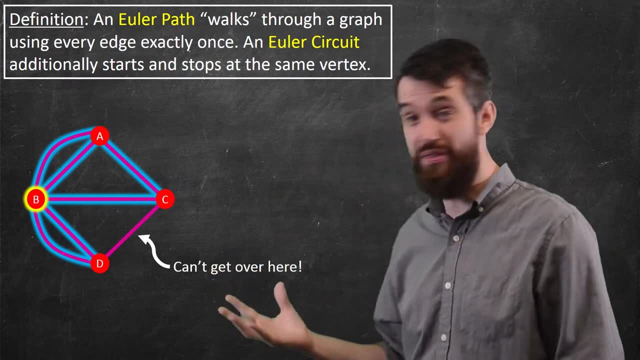 So in this particular graph at least, the path that I chose. I wasn't able to go and do everything once. Now you can pause the video if you like and see whether you can find some path that gets through here. that does hit everything. 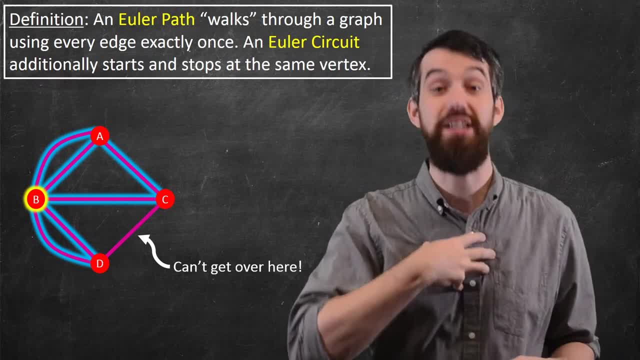 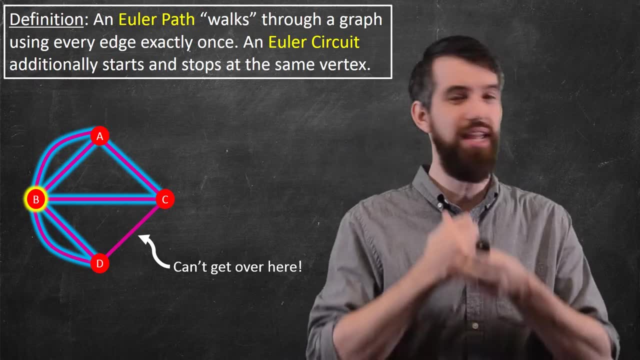 But even if you don't get a path- and I didn't get one when I tried to do it- that maybe there's still somebody out there who's creative enough that could find one. So is it impossible? Well, it turns out it is impossible, and we're going to use a little theorem about Euler. 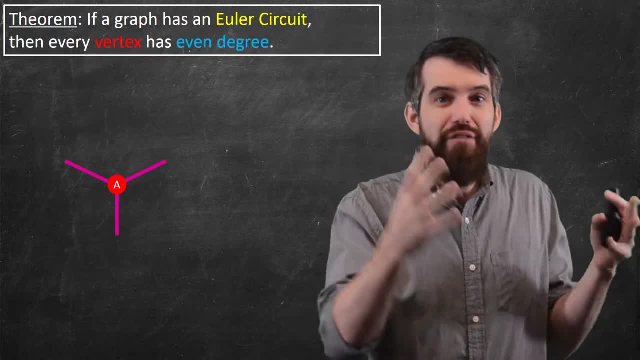 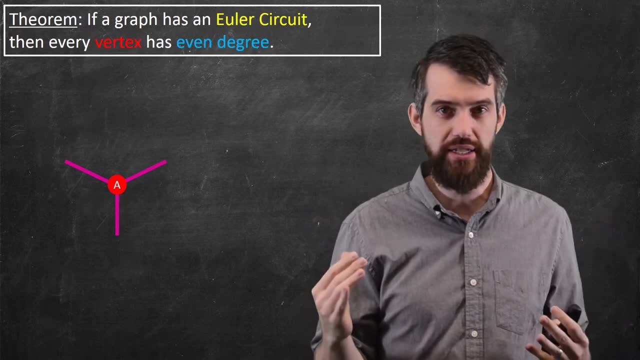 circuits, And the theorem says this. It says that if you have a graph with an Euler circuit, so one that starts at a vertex, goes around, gets back to the same place and hits every edge once, well then every vertex in that graph must. 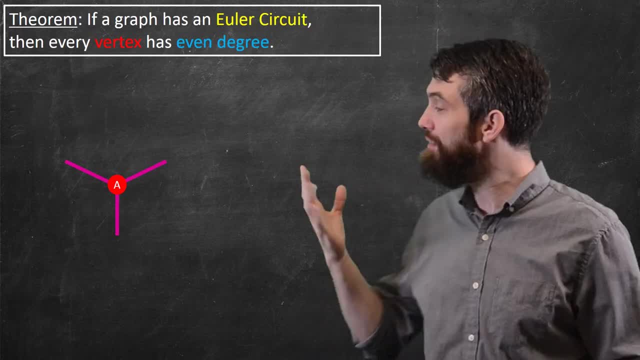 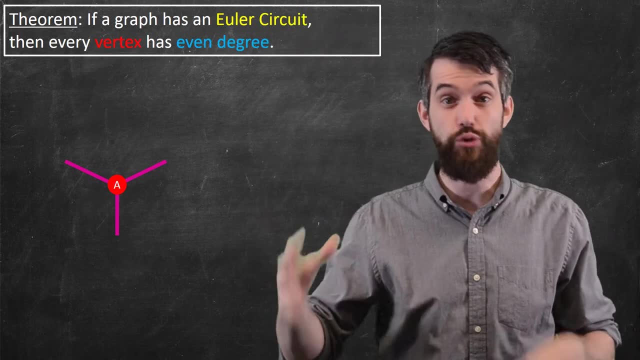 have even degree. Why is that true? So I've given a little small portion of the graph. It's got a vertex and it's got edges leaving it, And this is not a graph by itself. It has a whole bunch of other vertices around there, but I'm just not showing them. I'm 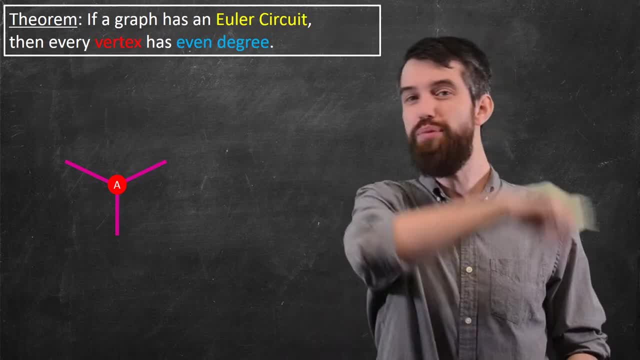 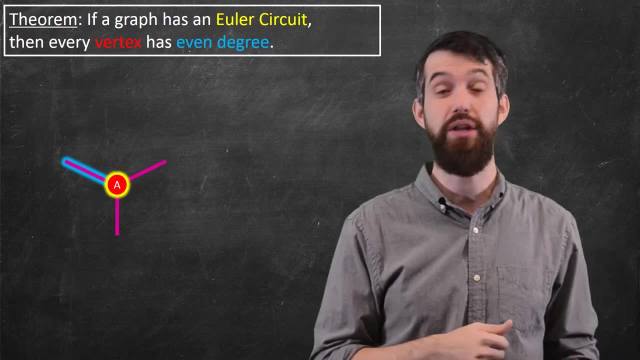 just going to zoom in on this one vertex. So imagine that I'm going through, I'm doing my Euler circuit and I get to this particular vertex A. So I come in and maybe go along from the top left and I hit out this value of A. Okay, so I've got to the A. Now I have. 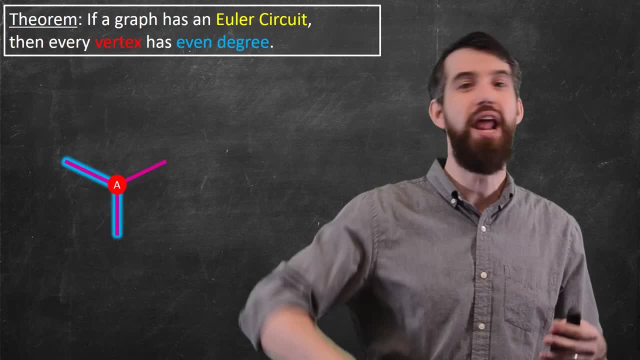 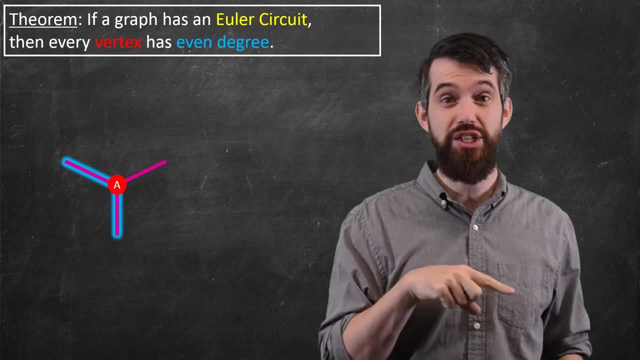 to leave. so maybe I'll go out the bottom here, So I leave and then I go off and do a bunch of other stuff in the graph, Who knows. But eventually, because I want to hit every one of these edges, exactly one time I'm going to have to come back in and I go in and get 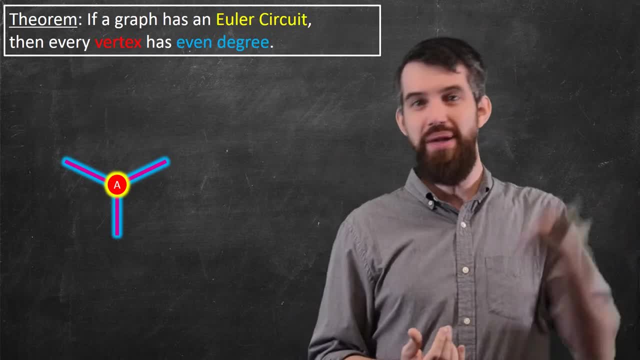 to A again. But now I'm standing on A, I've come in and I've gone out and I've come in again and now I'm on A and I can't get out. I'm trapped. If I want to leave A, I'd have. 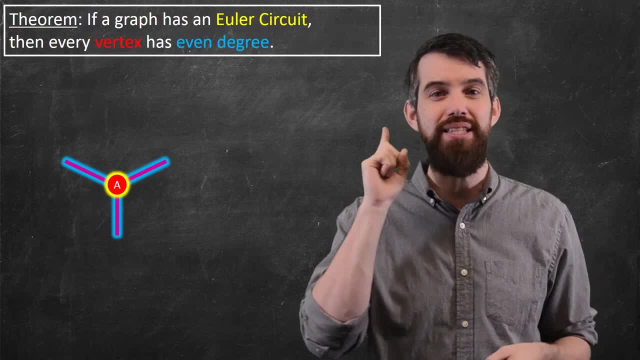 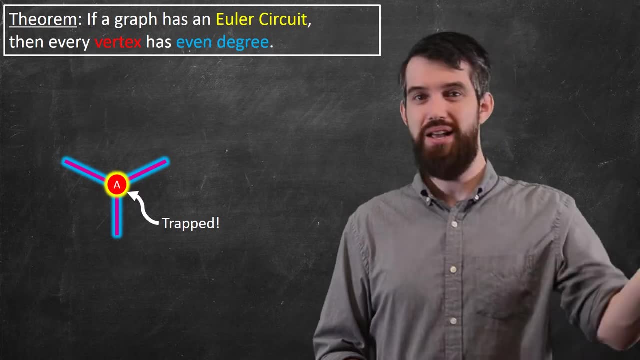 to leave an edge that I've already covered, So I can't hit it exactly once, And indeed, whether it was 3 or 5 or 7 doesn't matter, as long as you can come in and go out, come in and go out, come in and go out any number of times that you want to do this. 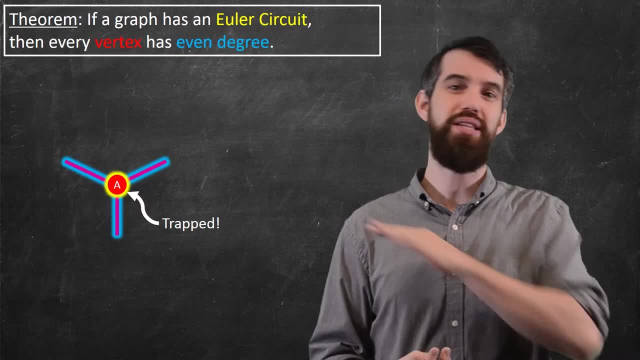 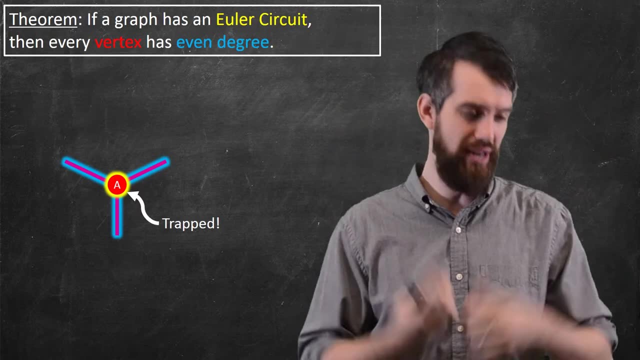 even property coming in and coming out, But if there's an odd number at some point, you're going to come in and you will be trapped and you will not be able to leave. And indeed this is even true if A is your starting vertex. right, Let's say you start there, okay, Well, 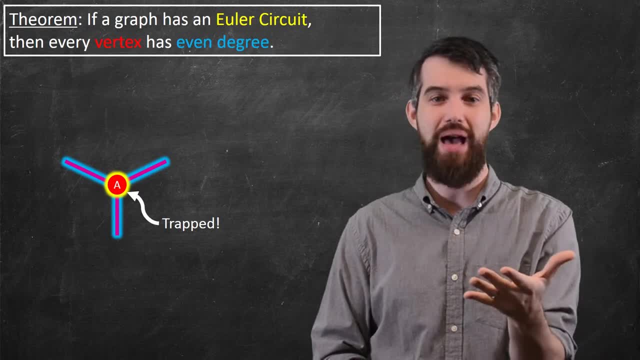 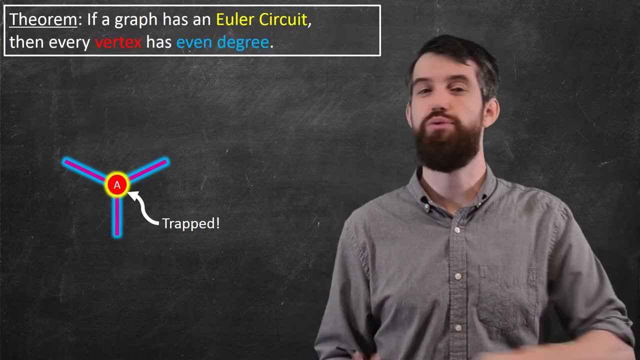 now you leave and come back, leave and come back, leave and come back. But if it's an odd number, eventually you have to leave and you will not be able to come back. And the fact that the Euler circuit that has to return to its origin is not possible. 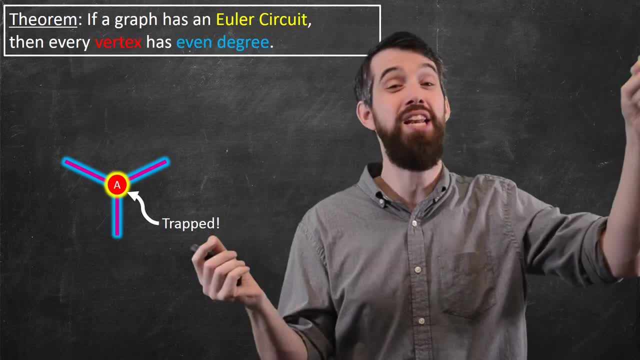 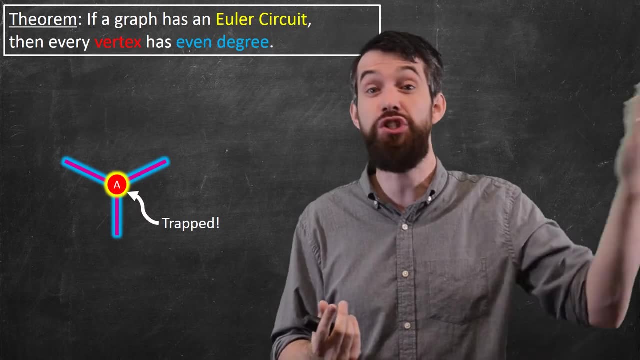 By the way, if you have an Euler path where you have a starting and ending vertex that are different, then the starting and the ending actually have to be odd, because your first is not a go and come back, it's just a go, And then everything else is going to be a. 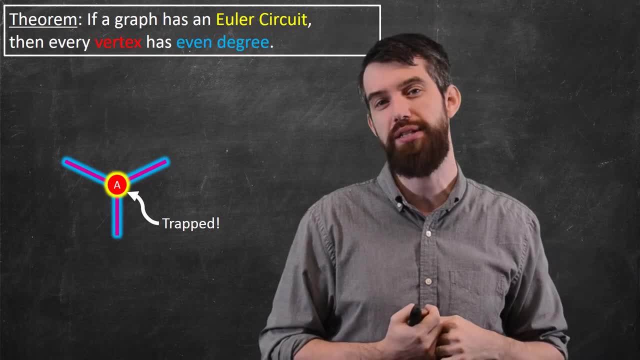 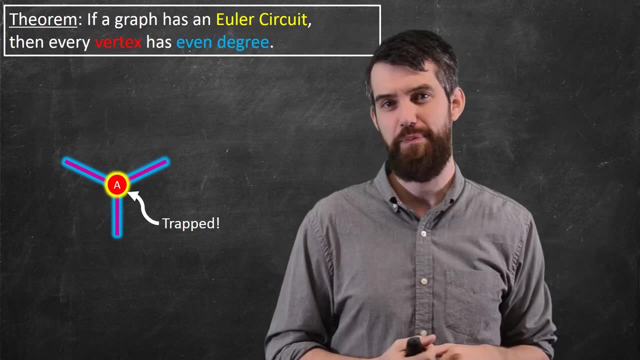 come back and go, come back and go, come back and go. if you're that starting vertex. However, all the ones in the middle do have to have an even degree to be an Euler path. Now I want to note that this is the statement of my theorem. it's an if-then and the contrapositive. 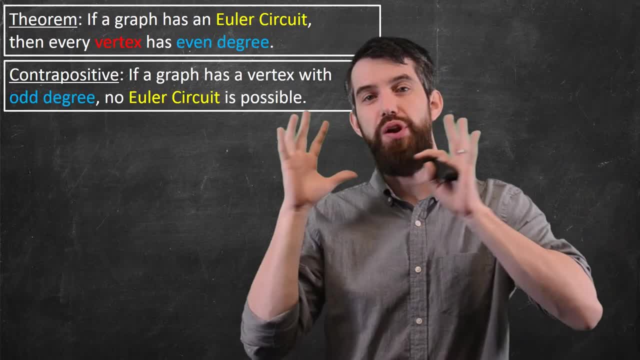 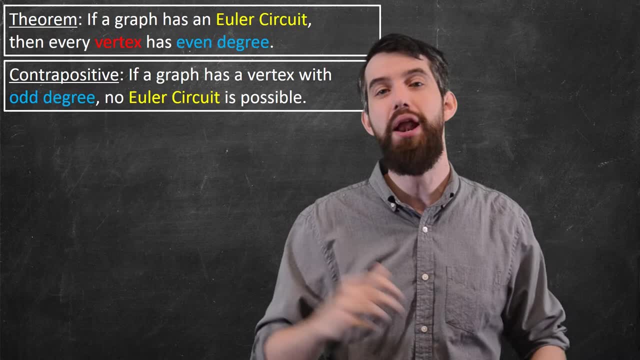 of that particular statement is that if you have a graph with an odd degree, any vertex at all, if there's even one vertex with an odd degree, then it's impossible, then you do not have an Euler circuit. So let's use that to study the particular graph that we.